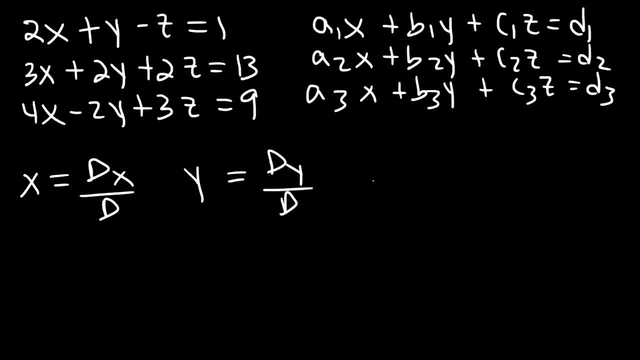 y is dy over d And z is dz divided by d. So we need to calculate dx, dy, dz and d, And then we can get the solution to these equations. So let's start with d. d is going to be a 3 by 3 determinant. 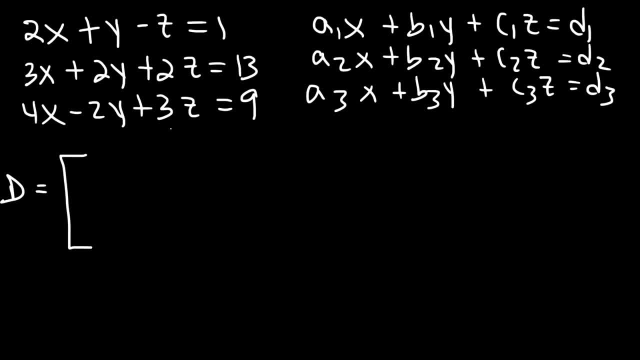 And the elements in this matrix is going to be a1, a2, a3.. So those are the coefficients for the x variables, And then b1, b2, b3.. So those are the coefficients for the y variables, And then c1,, c2, and c3., 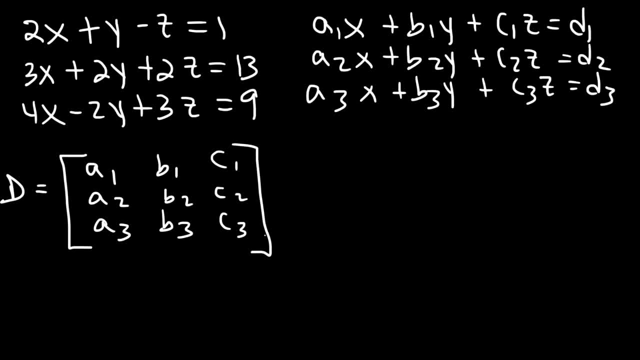 So you need to know how to evaluate a 3 by 3 determinant. So first let's start with a1.. If we eliminate row 1 and column 3, we'll get a3x and column 4.. We have aA5.. 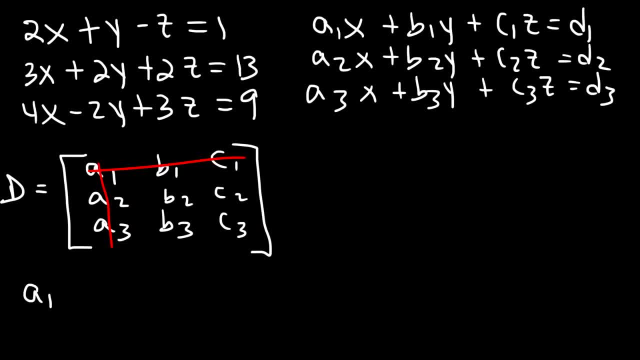 And we have a3x, column 1, we'll be left with this. So it's going to be A1 multiplied by a 2x2 matrix or the determinant of a 2x2 matrix, rather, B2, B3, C2, C3. 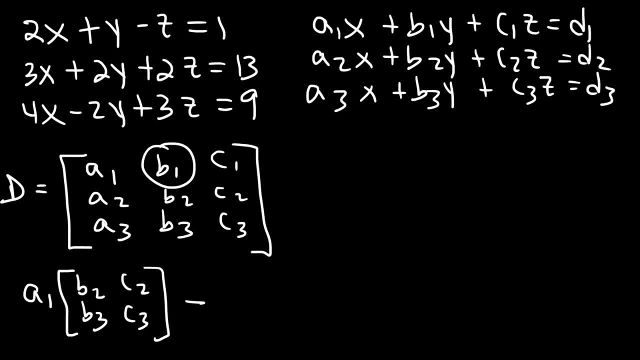 And then it's going to be minus the next one, which is B1, and we need to eliminate row 1, column 2, because that's where B1 is located, in row 1,, column 2.. And so we're going to have A2, A3, and C2, C3 left over. 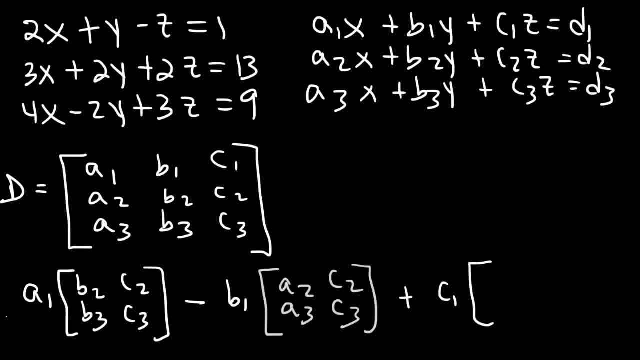 And then it's going to be plus C1, and C1 is located in row 1, column 3.. So we're going to get this Okay: A2, A3, B2, B3.. So that's how you can evaluate a 3x3 determinant. 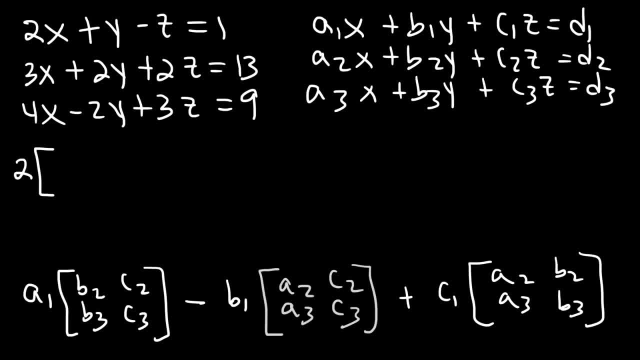 So in this example A1 is 2, and then B2 matches with 2,, so B2 is 2.. B3 is negative, 2.. B1 is 2, and C3 is 3.. And then minus B1.. 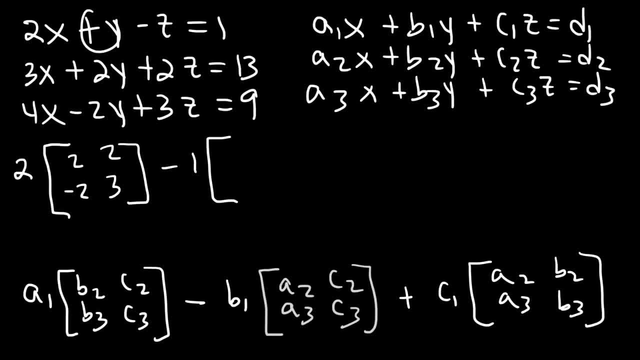 B1 is 1.. It's the coefficient in front of y, And then A2 is 3.. A3 is 4.. C2 is 2, and C3 is 3.. And then plus C1,, which is negative, 1.. 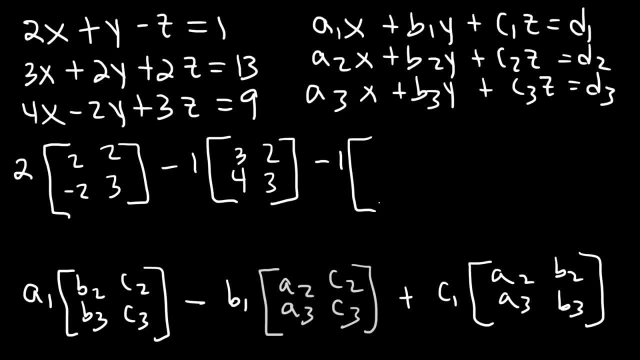 So C1 is in front of y, And then C1 is in front of z. That's negative 1. And then A2, that's 3, A3 is 4. B2 is 2, B3 is negative 2.. 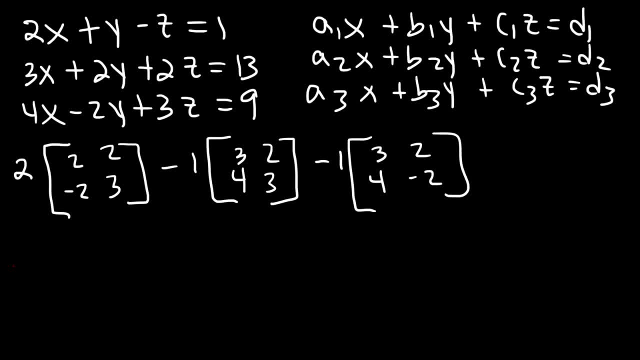 So now let's find the determinant of a 2x2 matrix. So it's going to be 2 times 3.. And then minus 2 times negative 2. And we still have a 2 in front of that. This is going to be 3 times 3,, which is 9,, minus 2 times 4,, which is 8.. 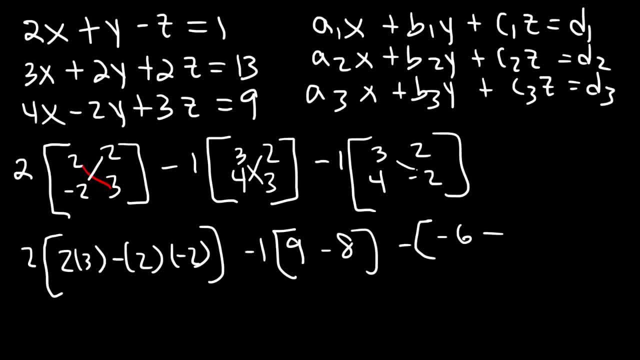 And this is going to be 3 times negative, 2,, which is negative, 6, minus 2 times 4,, which is 8.. Now, 2 times 3 is 6.. Negative 2 times negative 2 is positive 4.. 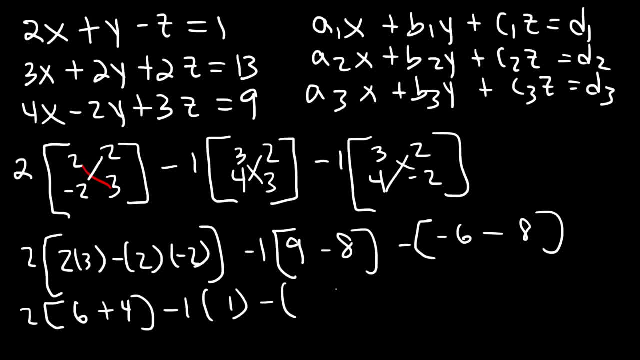 And 9 minus 8 is 1.. Negative: 6 minus 8 is negative 14.. 6 plus 4 is 10, times 2 is 20.. And negative negative 14, that's positive 14.. So we have 20 plus 14, which is 34, minus 1, that's 33.. 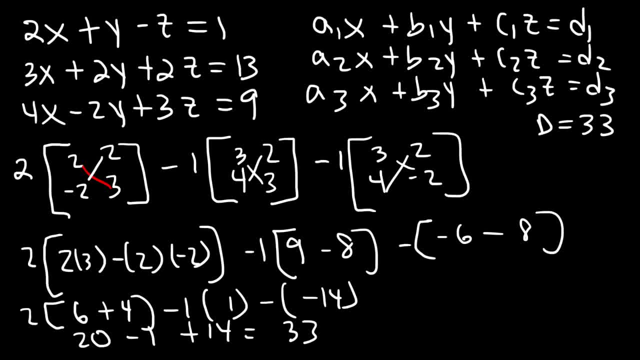 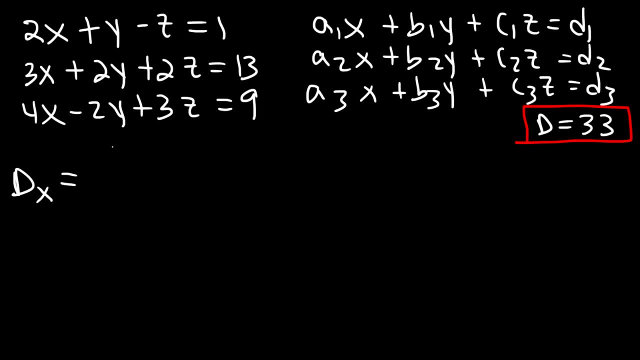 So d is equal to 33.. Now let's calculate dx. So for the elements in dx, replace the coefficients in front of x with d1, d2, d3. So it's going to be d1, d2, d3, and then b1, b2, b3, and c1,, c2, c3.. 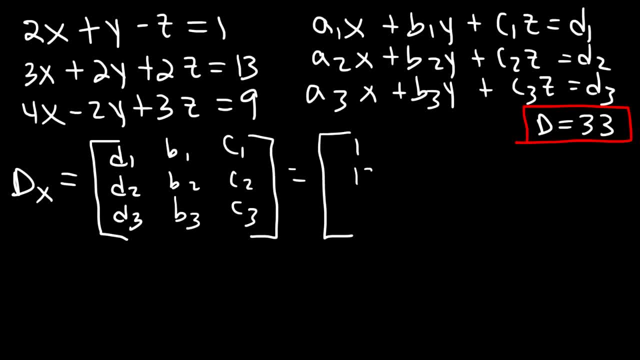 So d1 is 1,, d2 is 13,, and that's 9.. And then for the b's, those are the coefficients in front of x, And then c1,, c2,, c3,, those are the coefficients for z. 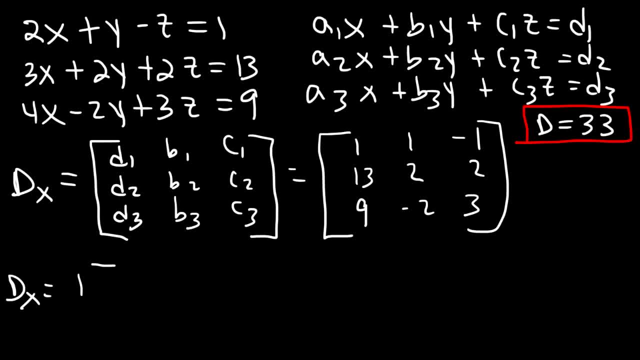 So we're going to start with this number. It's going to be 1.. And if we take out the row and column that correspond to that number, we're going to get these numbers. So that's 2, 2, negative 2, and 3.. 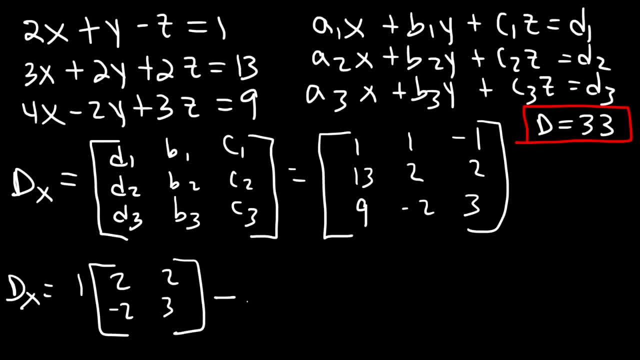 And then it's going to be minus the second one, Which is also 1.. And then that element corresponds to row 1, column 2,, leaving behind these four elements. So it's going to be 13,, 9,, 2, 3.. 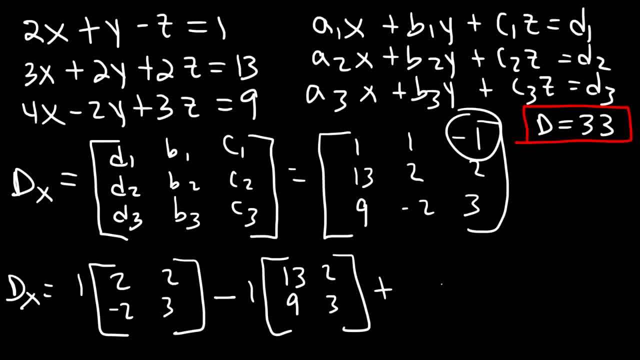 And then, plus this, one which is negative 1.. And that corresponds to row 1,, column 3., Which leaves behind 13,, 2,, 9, and negative 2.. So this is going to be 1 times 2 minus 3,, which is 6.. 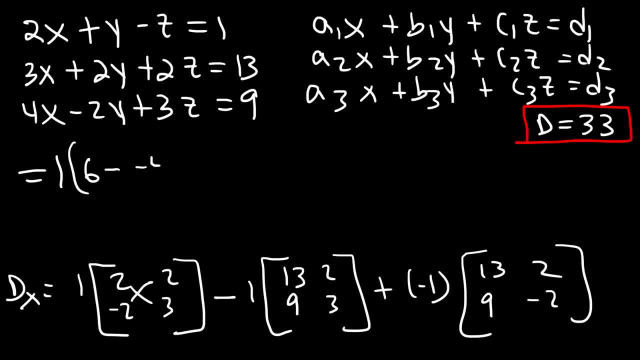 And then minus 2 times negative 2, which is negative 4.. And then it's going to be 13 times 3,, which is 39. Minus 2 times 9, which is 18.. And then 13 times negative 2,, that's negative 26,, minus 2 times 9, which is 18.. 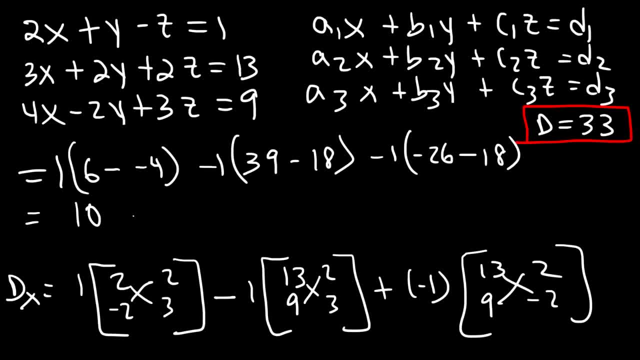 So 6 minus negative 4 is 6 plus 4, which is 10.. 39 minus 18 is 21,, with a negative 1 in front of it. so that's negative 21.. Negative 26 minus 18, that's going to be negative 44.. 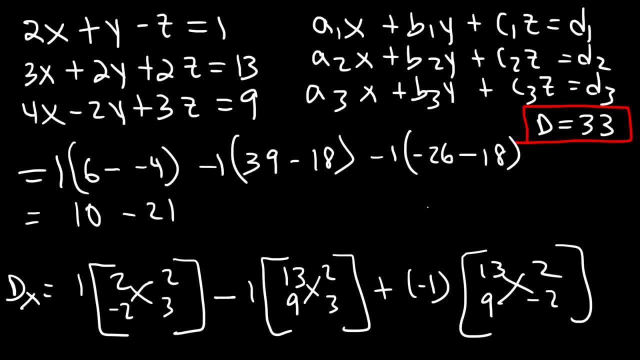 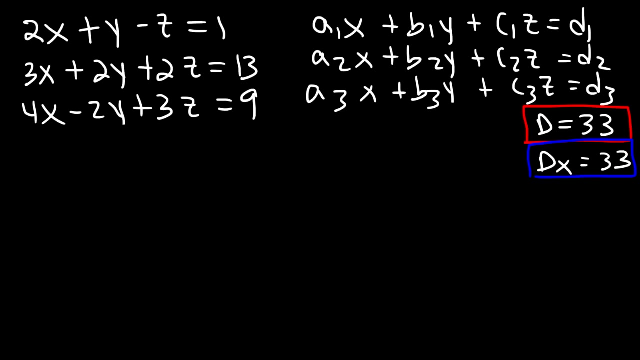 Negative 44. Times negative 1,, so that's positive 44. So we have 10 plus 44,, which is 54,, minus 21,, which is 33.. So dx is equal to 33.. Now let's focus on dx. 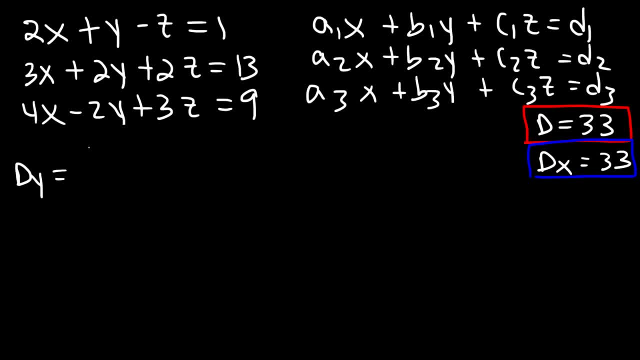 So this time the coefficients in front of y, we're going to replace it with d1, d2, and d3.. So it's going to be a1, a2, a3, and then d1,, d2, d3, and then c1,, c2, c3.. 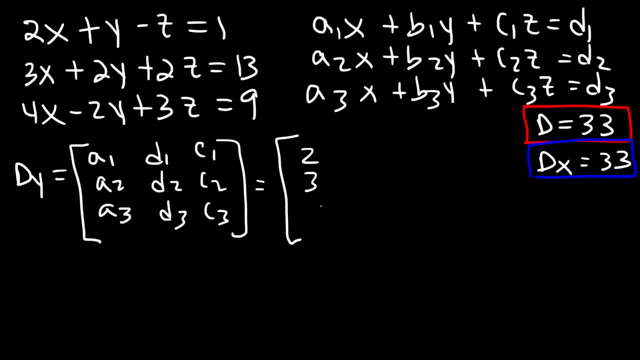 So this corresponds to the numbers 2,, 3,, 4.. 1,, 13,, 9, and negative 1,, 2, and 3.. So let's start with this number 2.. So that's in row 1,, column 1.. 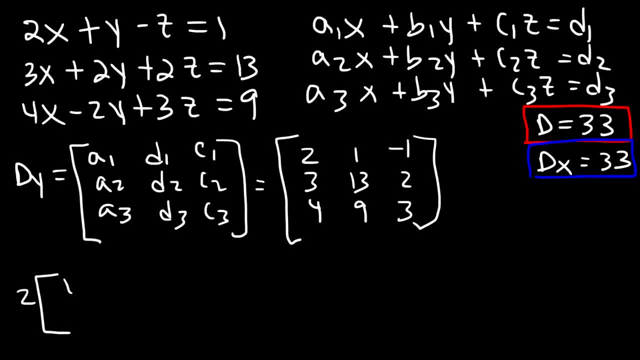 So it leaves behind 13,, 2,, 9,, 3.. And then minus the next number, which is 1.. And that's located in row 1,, column 2.. So it leaves behind 3, 2.. 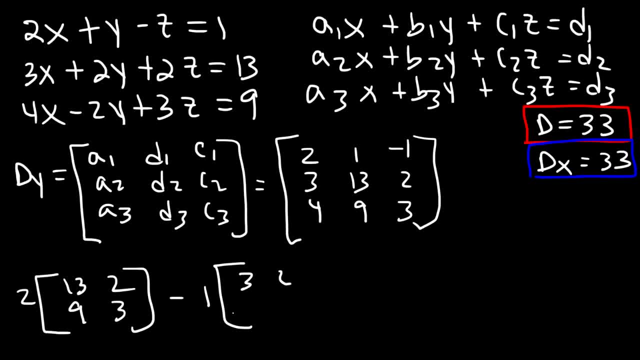 2,, 4,, 3.. And then it's going to be plus negative 1, and that's in row 1,, column 3.. So that's going to be 3, 13,, 4, 9.. 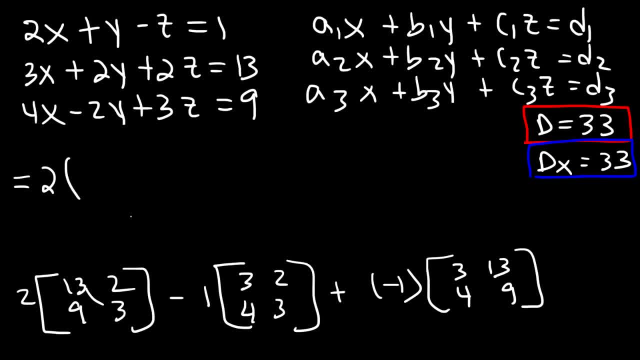 So this is going to be 2.. And then 13 times 3 is 39. Minus 2 times 9,, which is 18.. And then 3 and 3 is 9.. 2 and 4 is 8.. 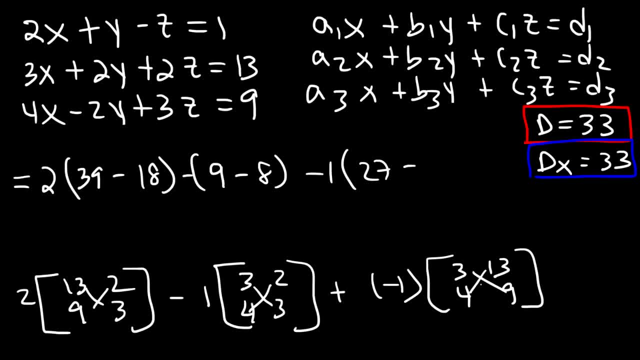 3 times 9 is 27.. 13 times 4 is 52.. Now, 39 minus 18 is 21.. 9 minus 8 is 1.. 27 minus 52,, that's negative 25.. 2 times 21 is 42.. 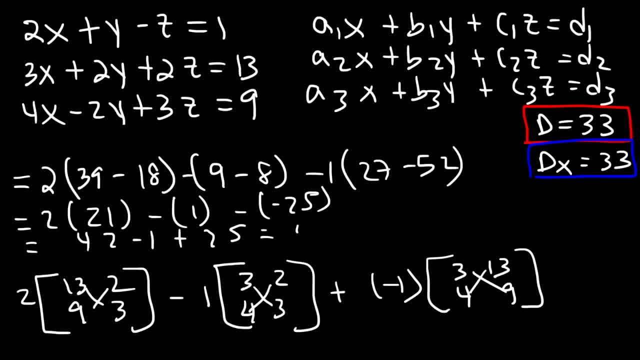 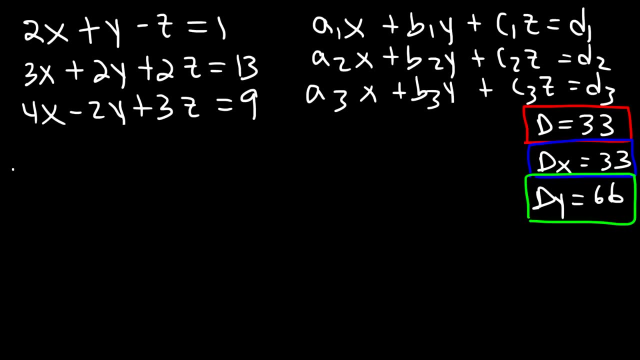 And 42 minus 1 is 41.. 41 plus 25 is 66.. So dy is 66.. Now let's move on to the last one, dz. So in this case the coefficients of z will be replaced with d1,, d2, and d3. 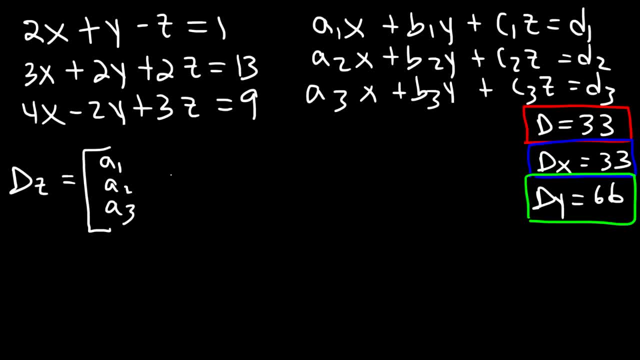 So it's going to be a1, a2, a3, b1,, b2, b3, and then d1, d2, d3.. So we're going to have the numbers 2, 3, 4, 1, 2, negative 2, and 1, 13,, 9.. 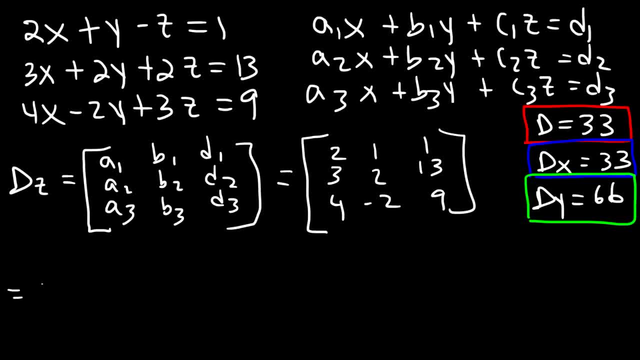 So let's start with this one: 2.. So if we eliminate row 1,, column 1,, we're going to have 2, 13,, negative 2, 9.. And then minus the next number, which is 1.. 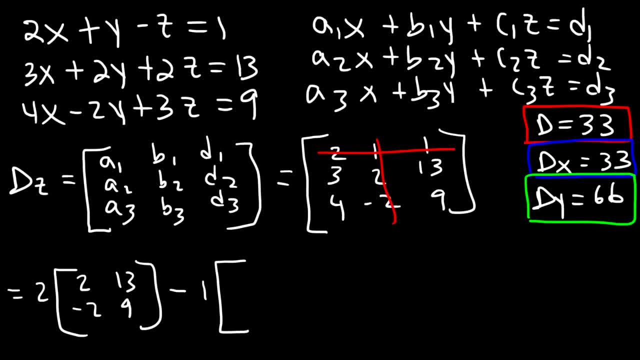 And then, if we eliminate row 1,, column 2, we'll have 3,, 13,, 4,, 9.. And then it's going to be plus 1.. So let's eliminate row 1,, column 2, we'll have 3,, 13,, 4,, 9.. 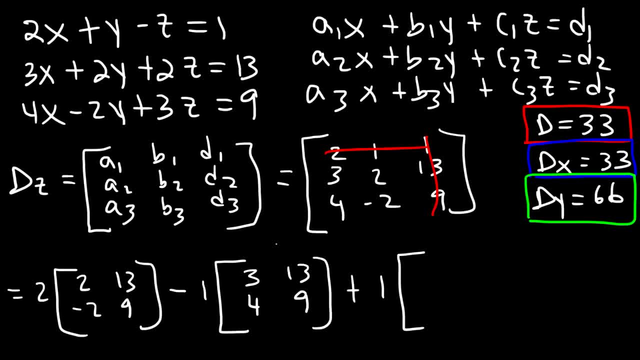 And then if we eliminate row 1,, column 3,, and that's going to be 3,, 2,, 4, negative 2.. So this is going to equal 2.. And then 2 times 9 is 18.. 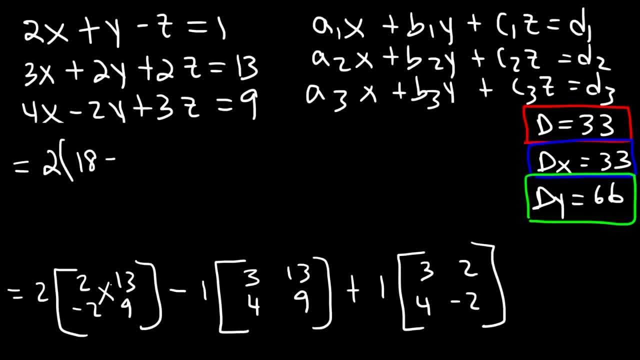 And then minus negative: 2 times 13,, that's negative 26. And then minus 1.. 3 times 9 is 27.. 13 times 4 is 52. And then 3 times negative: 2 is negative 6.. 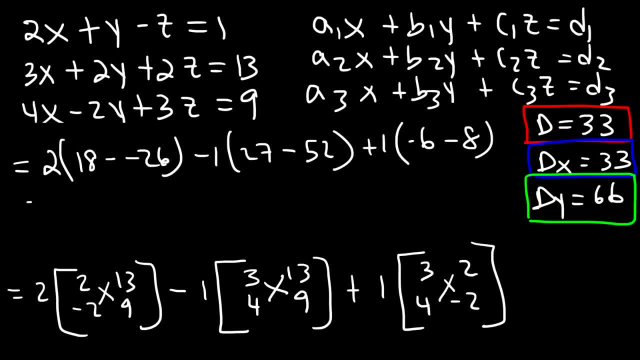 2 times 4 is 8.. Now 18 plus 26,, that's 44.. 27 minus 52 is negative 25.. And 6 times I mean negative. 6 minus 8 is negative 14.. 2 times 44 is 88..